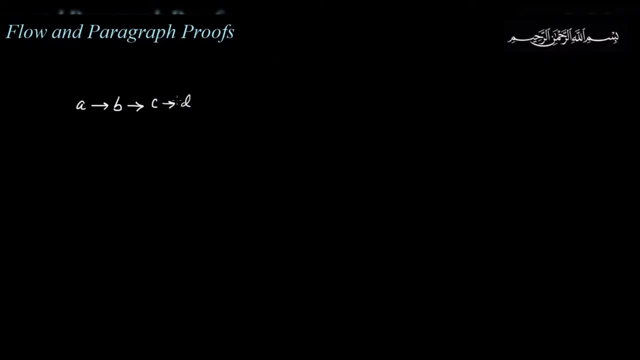 you have C and from there you have various different consecutive conclusions like this. So a deductive argument is a logical chain of statements linking an initial statement or given information and initial premise. Here I have labeled that as A. This would be the initial premise and from there you derive logical sequence of conclusions to: 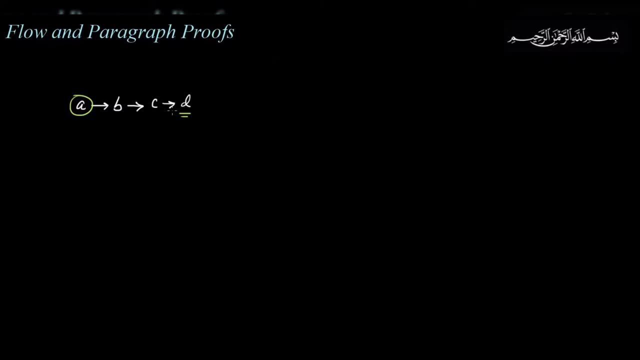 arrive where, at a final conclusion, And that, in this case, is D. A particular deductive argument can be one, two, three or hundreds of steps like this, if needs be. So this is an example of a deductive argument In geometry. we have different types of such deductive proofs or arguments, and you can 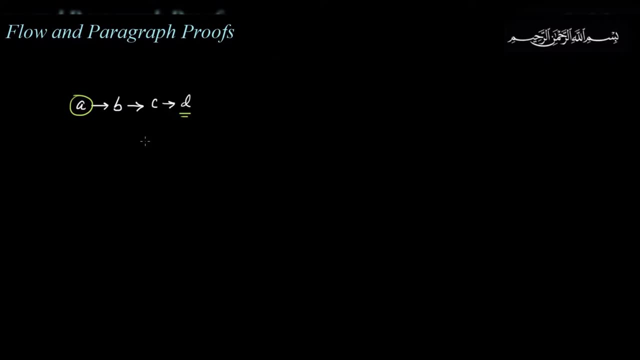 diagram them to allow people to understand your thinking more clearly. So proofs in geometry are of various different types. There are two that we're going to talk about today. Today we're going to talk about flow and paragraph proofs. In the future, we'll talk about a two column proof, which is in: 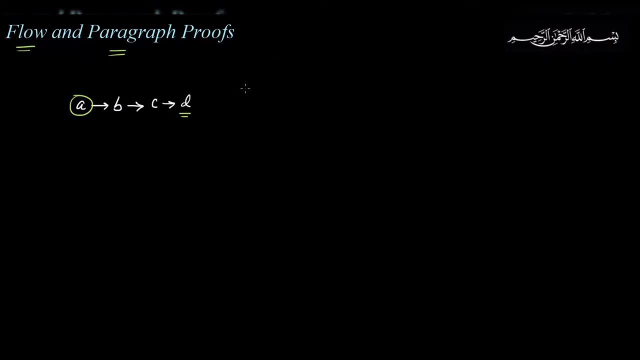 fact, the most common type of a proof that we're going to use. But today I shall introduce you to flow and paragraph proofs, But before we do that, I just wanted to review these concepts, these properties of real numbers that we talked about last time. So these are properties of 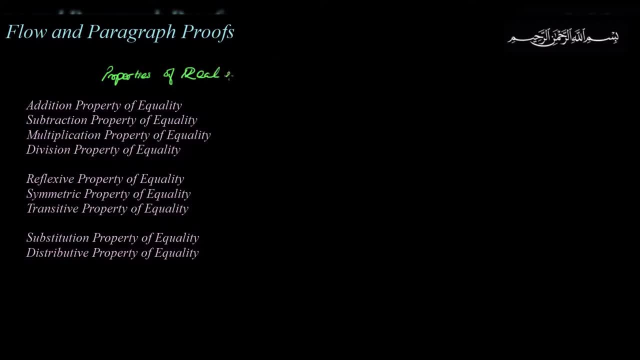 real numbers. Now, this is particularly important because these properties will show up in different forms in the future, so it's particularly important to know these really really well. So we had the addition property of equality for real numbers and subtraction property of equality, multiplication property of equality and division property of equality. That's 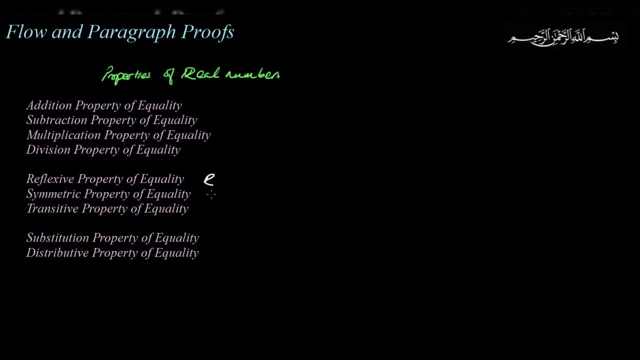 easy enough to remember, And then the reflexive property of equality, Symmetric property of equality, transitive property of equality and finally the substitution property of equality and the distributive property of equality. These are very, very, very important to memorize, in fact. 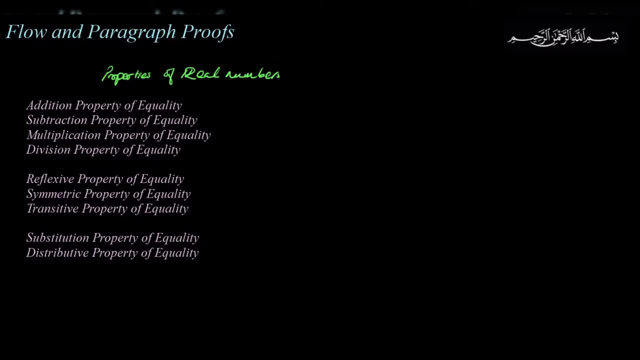 So you should be able to articulate these properties with reasonable confidence, like this Addition: property of equality is that if A is equal to B- and this is for real numbers- A is equal to B. if a is equal to B, you can simply just put this as an error. then A 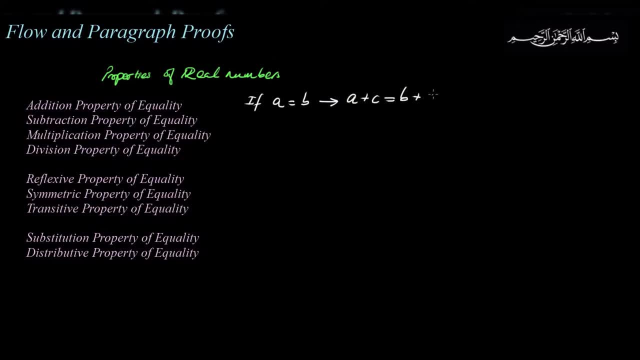 plus C is equal to b plus c. Now you can write this in a sentence form this way: if A is equal to b, then A plus c is equal to b plus c. That's the addition property of equality. Subtraction property of equality is very similar, of course. if A is equal to b, then A minus. 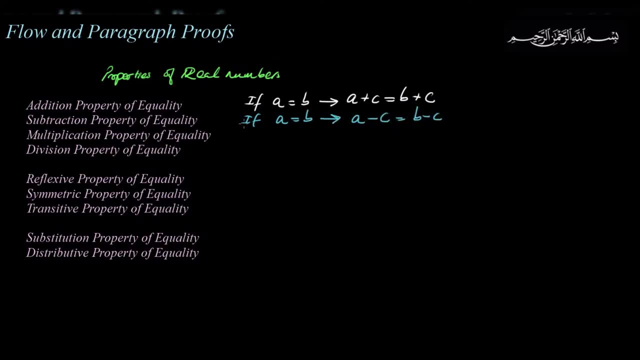 c is equal to b to b minus c. In a similar way, the multiplication property of equality- if a equals b, then a times c is equal to b times c. And finally, the division property of equality says: if a is equal to b, from this will flow that a divided. 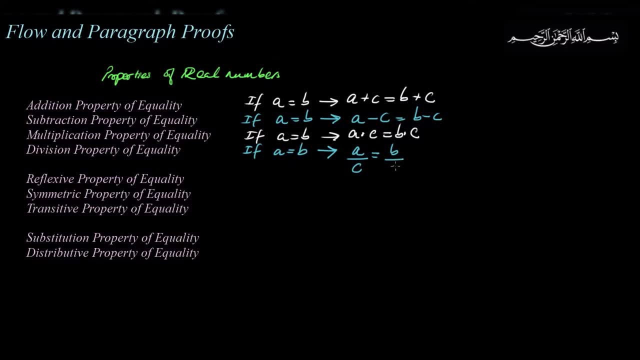 by c is equal to b divided by c. And here, if you recall, we must add that c cannot be 0, because division by 0 is not defined. So this is a very important fine print, so to speak, or a proviso, for this particular property. So addition: 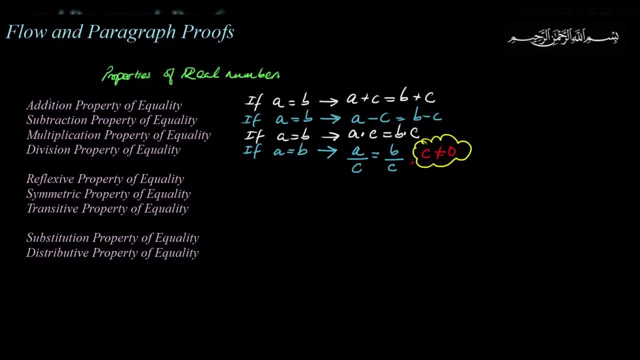 property of equality states that if a equals b, then a plus c equals b plus c, And the subtraction property, multiplication property and division property are very similar in conceptually as they are written Now. these others might seem very simple or basic to you, but they're very important. 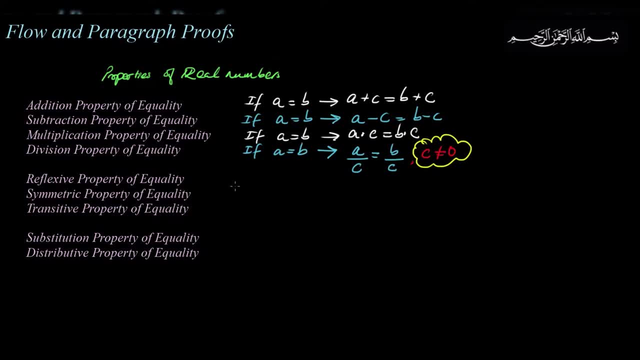 and very useful. Reflexive property of equality says that a number- in these cases, these are all properties of real numbers. In reflexive property of equality it says a number is equal to itself. a is equal to a. Now, symmetric property of equality is: 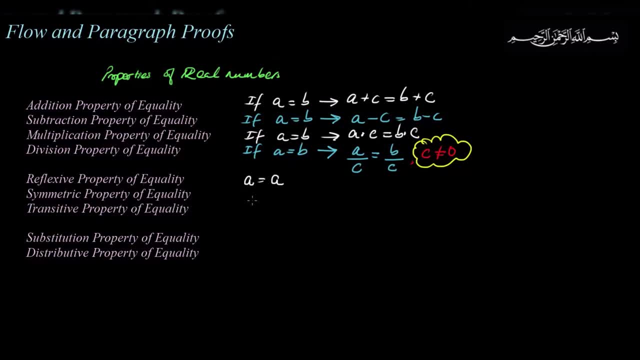 slightly different. see Symmetric property of equality says: if a is equal to b, right, then b is equal to a. In other words, you can like flip these around like that: If a is equal to b, then b is equal to a. I'm using these errors to substitute for the. 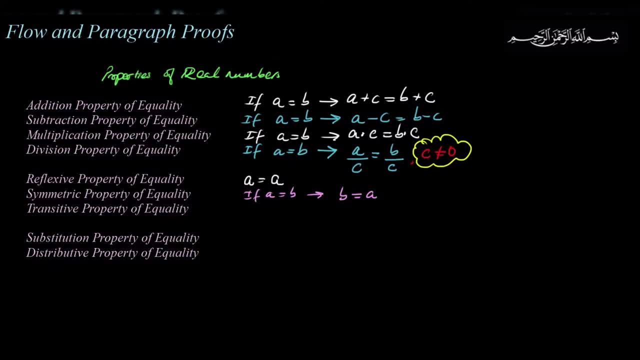 word, then, because I just find it's just easier to write it that way: If a equals b, then b equals a. The transitive property of equality is perhaps one of the most often and commonly used and states that if a is equal to b, 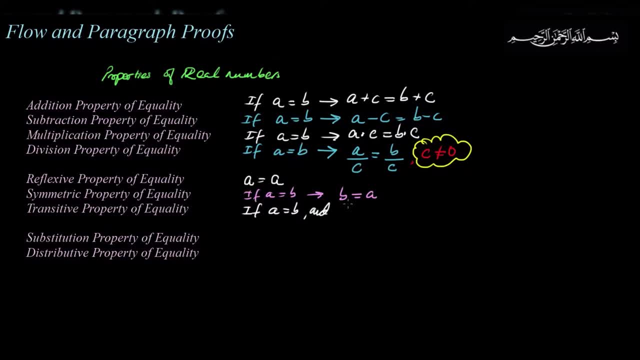 alright, and b is equal to c, then a is equal to c. If a is equal to b, b is equal to c, then a is equal to c. So in transitive property of equality you have to understand that you have to have something common, a bridge, If a has to go. 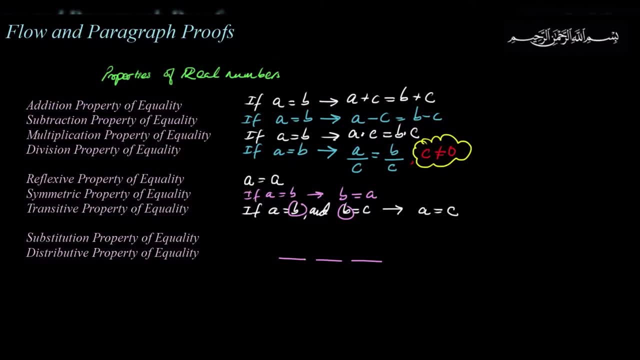 to b and b has to go to c so they have to overlap. So a equals to b and the b equal to c. they have to overlap like this to be able to use the transitive property. If a equals b, a equals b and b equals c, then you can say that a and c are related. a equals to c. 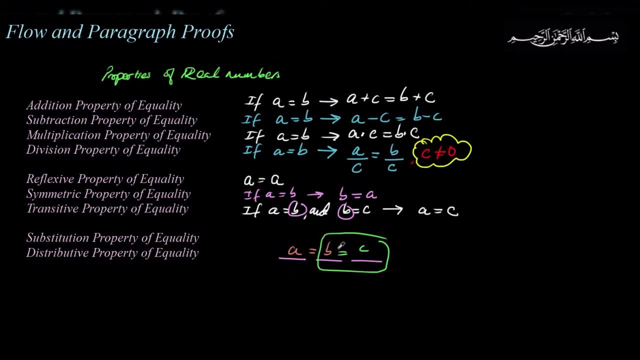 like this. So that's the transitive property of equality, and it's very important to be able to articulate that one as well. And finally, substitution property of equality says that if a is equal to b, then a may be replaced by b in. 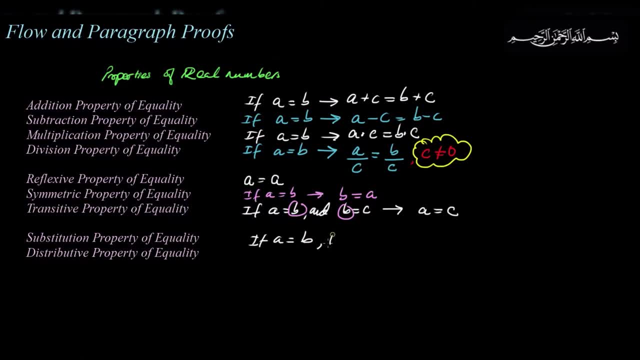 any equation of expression. If a is equal to b, then I'll use my arrow again. then a can be, let's say, n. it can be replaced or substituted for b in any expression or equation. Now, these are all properties of real numbers. okay, So if a is equal to b, 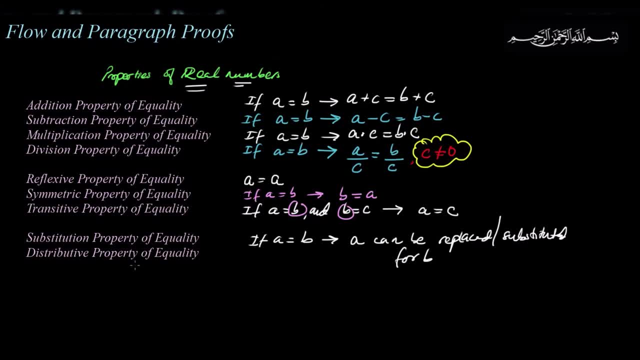 then a can be replaced, substituted and finally, and if the distributive property of equality- you probably also are familiar with this- a times the quantity B plus C. whenever you have parentheses, it's important to say that the word quantity, because then you say everything that follows after the statement. so eight times the quantity B. 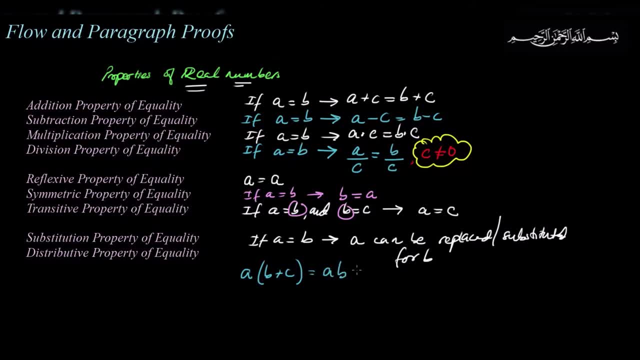 plus C is equal to a times B plus a times C, like this, alright. so addition property of equality, subtraction property of equality, multiplication property- we call a division property of equality- and then reflexive symmetric transit property of equality, substitution and distributive property of equalities. it is imperative to know these extremely well because, as I said, 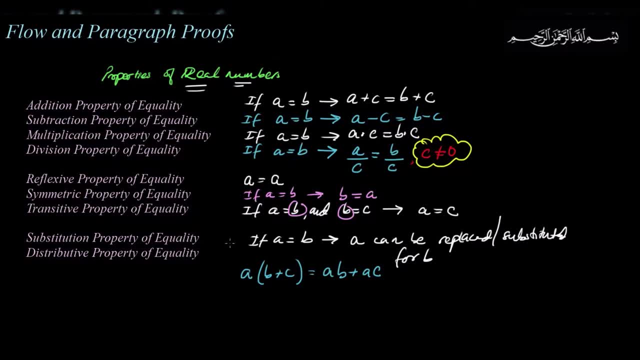 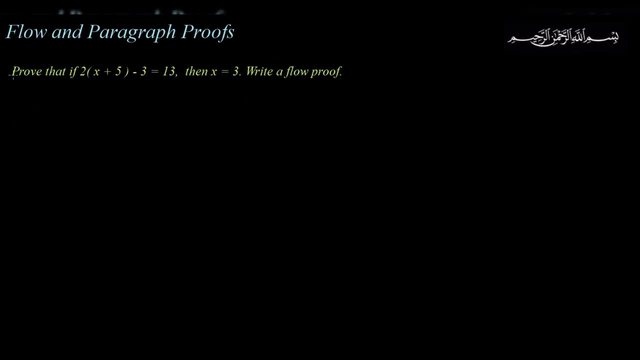 these will come again and again in various different forms. okay, so here's an example of a flow proof. so here we asked here: chat, prove that if 2 times the quantity of X plus 5 minus 3 equals 13, then X is equal to 5, and we're asked here to write. 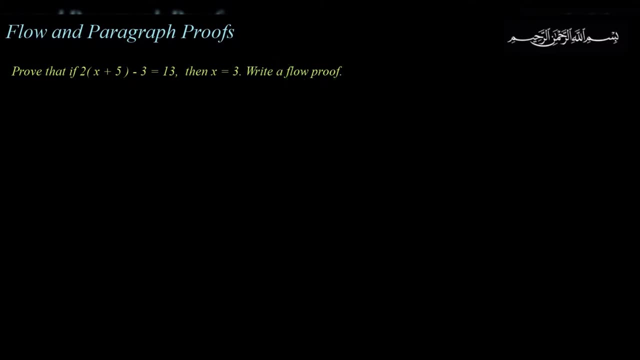 a flow proof. so what is a flow proof and how do we go about writing a flow proof? a flow proof is basically diagramming. you steps. you start with the given information and you go through basically a series of deductive conclusions like this, and at each step you provide your reason. so you start with the given. 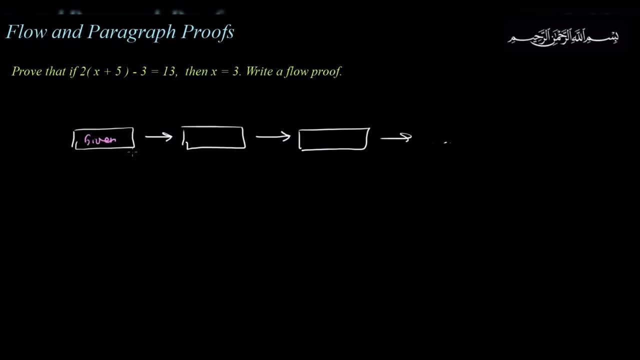 information over here and you manipulate that information into logical reasoning and get the information that we have to come up with certain conclusions to the eventual result, in to what you are trying to prove, that which you, that which you have to prove. in this case, you want to prove that X is equal to 3, so you 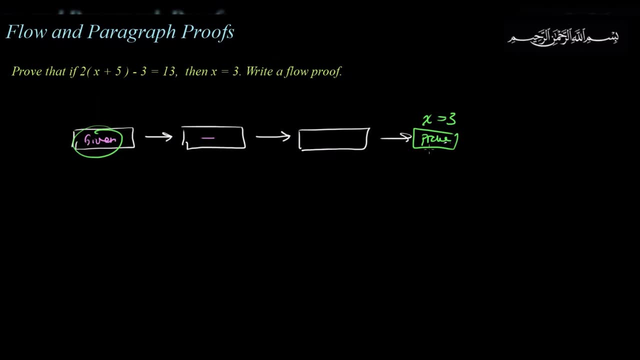 start out with given information and you come to the conclusion over here, or whatever you're trying to prove, through a series of step, and what you do is you, you draw a diagram like. then you can retangulate each particular step to make it look prettier, and then you provide each reason below. so reason for every. 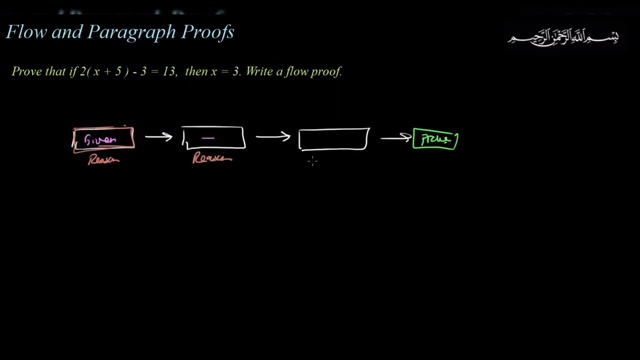 step is given like this. so reason for this, reason for this. so reason for this step is over here. reason for this step is over here. except for whatever you do, you have to provide a reason like this: okay, there may be more steps in this particular proof than- and then here. so this is an example of a flow proof and 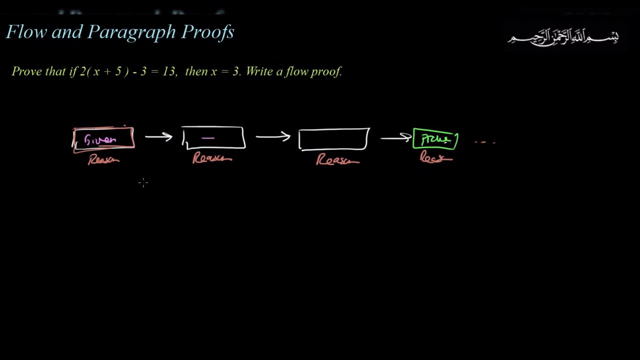 flow proof basically diagrams you thinking and forces and requests you or requires you to write the reasons behind every particular step. so the first thing you do in a flow proof is that you write the given information and you write what you have to prove. so in this case, we are given the this particular equation. so 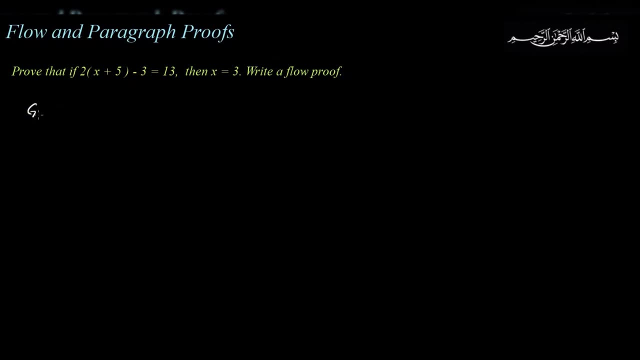 let's write that as a given information. so we are given that 2 times the quantity X plus 5 minus 3 is equal to 13. that's what's given and we are required to prove. if that is given, then we are asked to prove that X is. 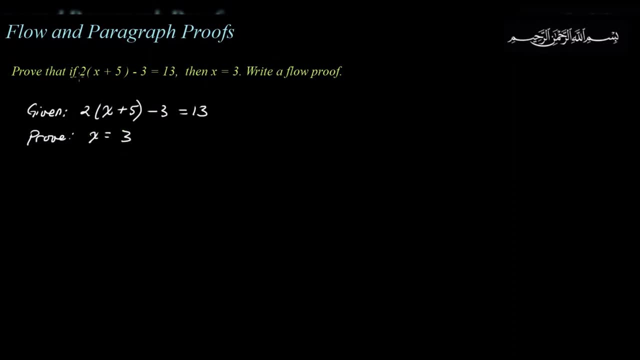 equal to 3. so the first step in writing a flow proof is to write the given and information and what we are required to prove, and then we write the flow proof. here is the the flow proof. so a winning doubt. it's a good rule of geometry just to actually start from the given information. that's generally. 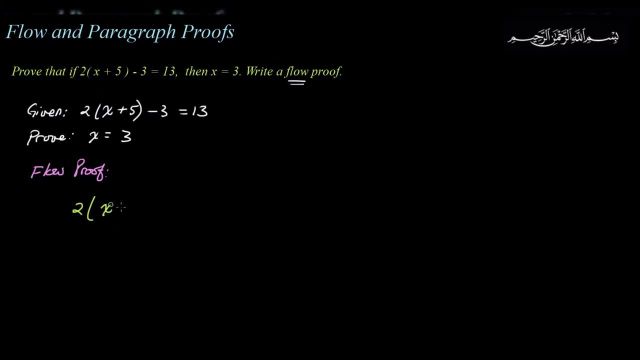 where you always need to start anyway. so 2 times the quantity X plus 5- okay, minus 3- is equal to 13. so you start out with the given information and here I am going to kind of. this is what I call this, the rectangle eating, and putting them in a 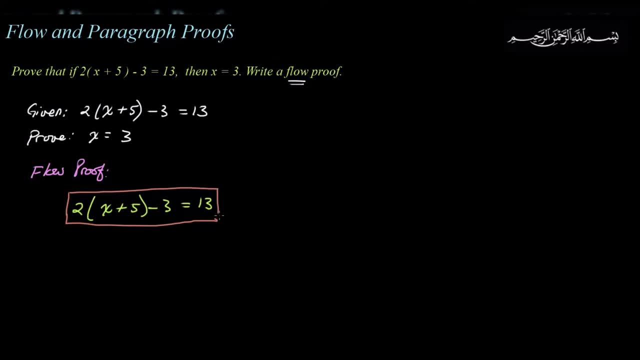 box like this, and this is so simply to make it aesthetically appealing to the reader. and you know it's there's no law, that you have to do this and you make a square rectangle, but the time makes it neater. so this is, this is what's given. 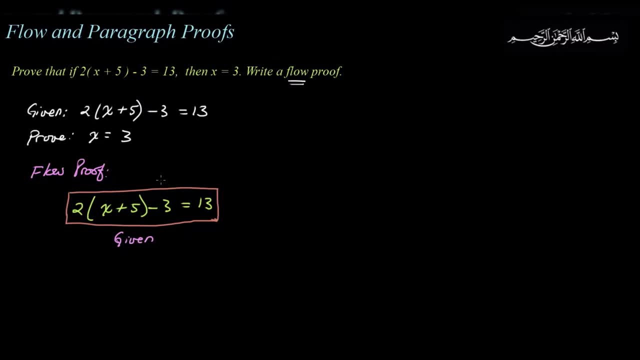 to us. so the first step is that that's a given information. all right, now, basically, you're solving the equation, but then you have to give a reason for everything that you do well in solving this equation. the first thing that I'm going to do is I'm gonna add three to both sides, like this: okay, so from 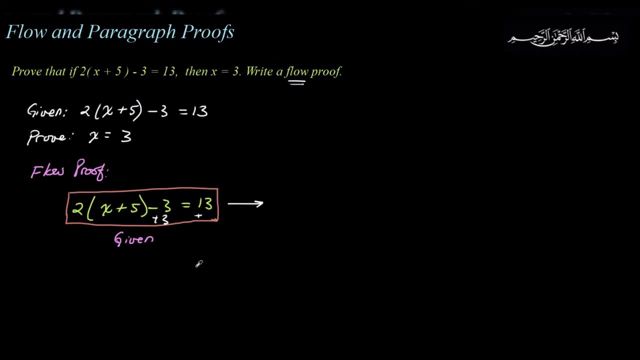 algebra we learned that that's kind of how you do things right, okay. so if you add 3 to both sides, what you are right, that is this: 2 times the quantity X plus 5, and then basically adding 3 to both sides, you get this is gone here, and then you get 16 right. so you get 16, so that's. 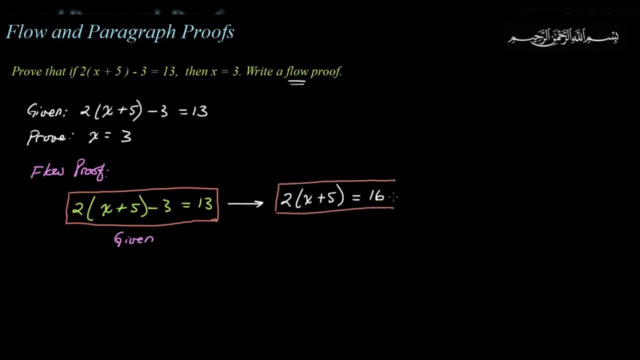 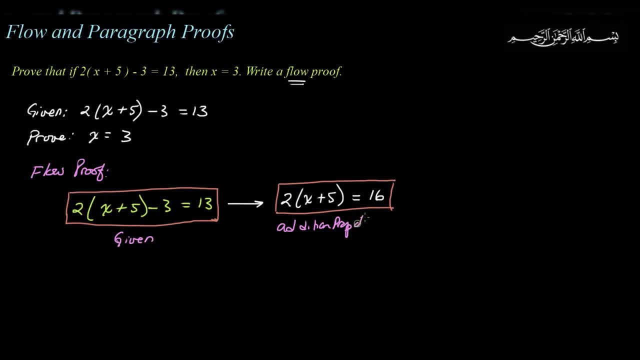 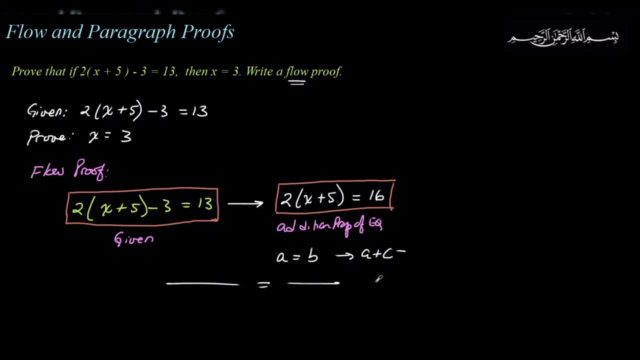 be okay. so that's the addition property of equalities. the reason for this step being a legitimate step, the reason we can say this over here like this, is because of the addition property of equality. so let me write that down. so: addition property of equality. so for 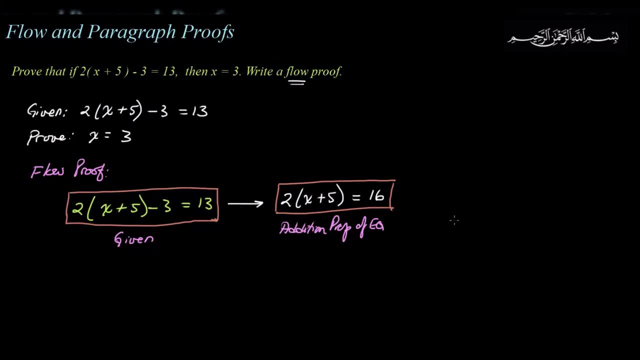 real numbers. it is all real numbers. we are assuming that here. so, and then, what do you do next? well, in, if you wanted to solve this, we can do couple ways. actually, you can actually distribute this right. right, that's one way of doing that, and that would be okay too, because in algebra there's more than one way of. 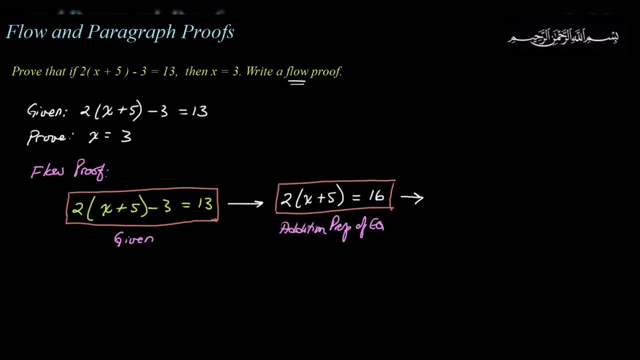 solving equations correct. but here I'm going to divide both sides by 2, like this see. so I can divide both sides by 2, and if you do that, on the left side you have X plus 5, and then it's going to equal to: if you divide 16 by 2, you get 8, okay, so 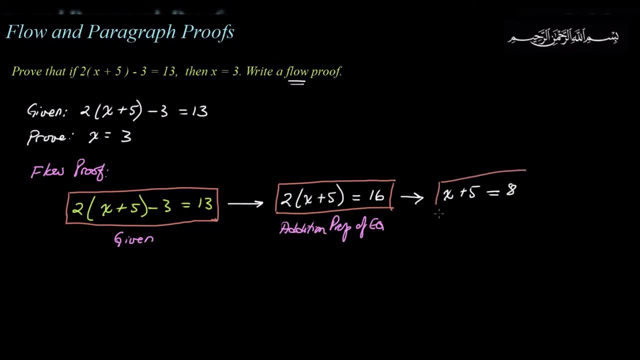 that's pretty good. now, what's the reason that I can do that? why is it? why? why is it legitimate? why it for me to do something like that correct? well, it's legitimate because of the division division property of equality, right? because the division property we call it says: if a is equal to B, then a divided by C is equal to B divided by. 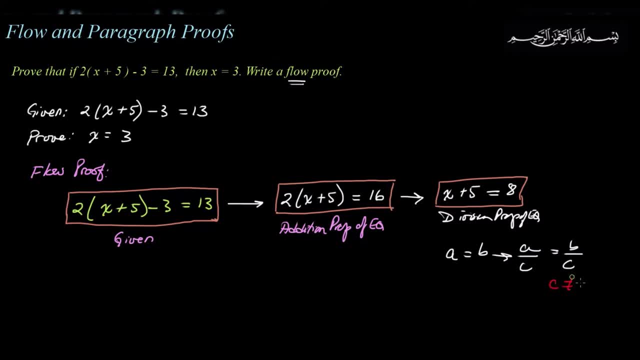 C, provided that C does not equal to 0, and clearly C is not 0, because here you're dividing by 2, so this step is very legitimate and I can do this because of division, division, property of equality. and finally, I can subtract 5 from both sides. 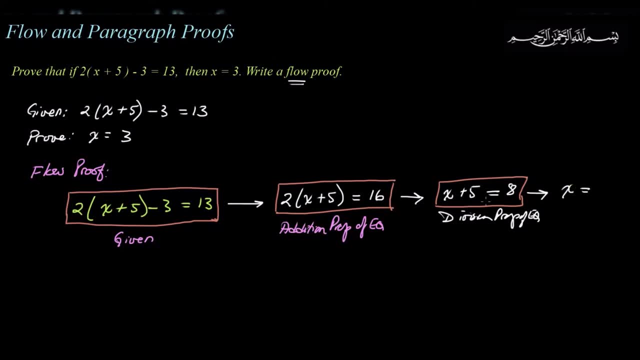 and I can get: X is equal to subtract 5 from both sides of the equation and X is equal to 3 over here, like this right. so, and what is the rationale for this? well, there's a reason why I reviewed on all them properties here and the rationale. 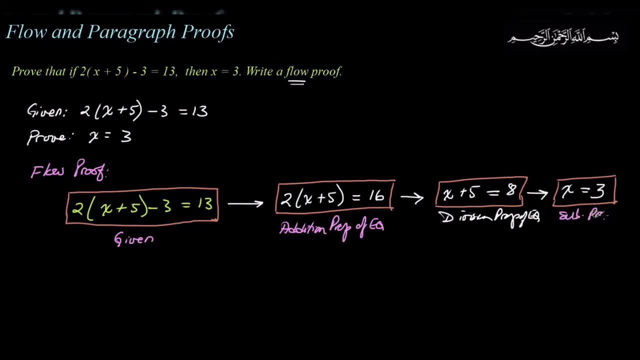 for that, of course, is subtraction property of equality for real numbers, because subtraction property of equality says that if a is equal to b, then a minus c is equal to b minus c, like this. okay, so, and hence we have proven that, that if this given information is true, then we 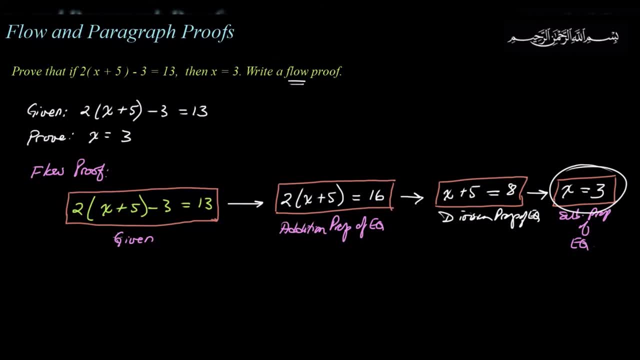 can arrive at this particular conclusion: that X is equal to 3, right? so? and this is an example of a flow or a paragraph proof. so in a flow of a paragraph proof, a flow. sorry, this is an example of flow proof. in a flow proof, you write the: 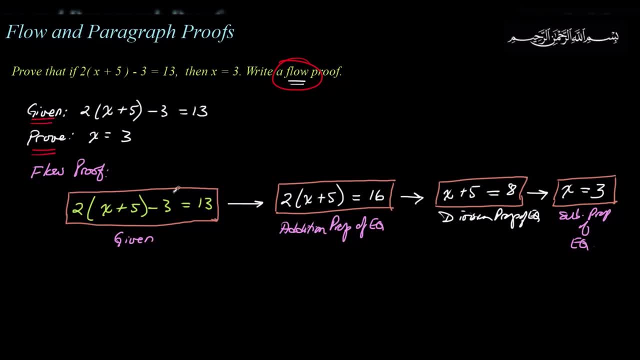 given information and you write what you're trying to prove and then you draw what's called a flow diagram like this in this case. this is an example of a algebraic flow proof, a lgb algebraic flow proof, because we're using basically algebra, solving algebraic equation. you can have geometric flow proof. 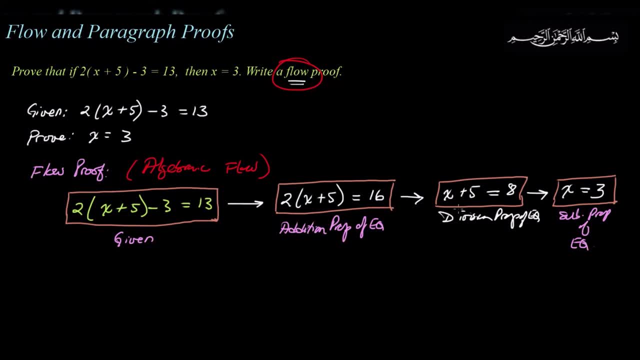 also, and which I shall show you in just a second. so, and then you, you draw what's called a flow diagram, flow proof. so you start with the given information and at each step you write why your step was justified or justified, and until you arrive at your conclusion. so this is one example of a flow proof. okay, so here is. 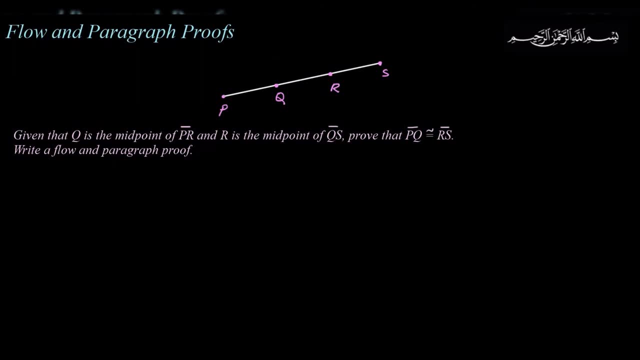 a geometric example. first let us read the question. the questions says that, given that Q is the midpoint of PR, so here's Q, and you're told that it is the midpoint of PR, segment PR right here. okay, that's the first point. so, given that Q is the midpoint of PR, and? and then you're told that R, which is here, is, 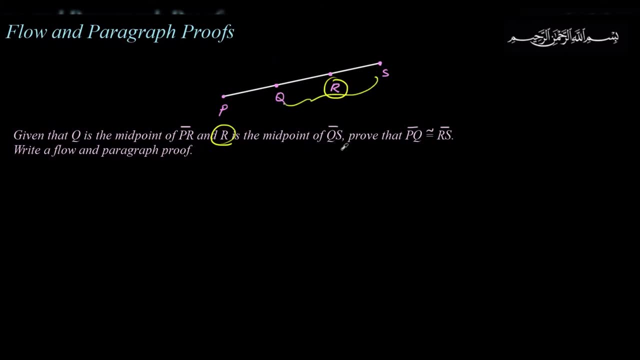 the midpoint of QS over here, and so if you're asked to prove that PQ is which is over here is congruent to RS over here, Okay so, and there are instructions are to write a flow proof and a paragraph proof here. So we're asked to actually to write the. 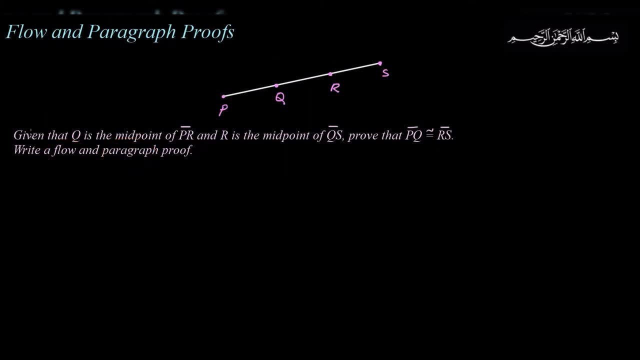 same proof in two different forms: and a flow proof, which is like a diagram proof, as we did last time, and the paragraph proof which I shall introduce to you next. So let's reread this question and see what we have. So, given that Q is the 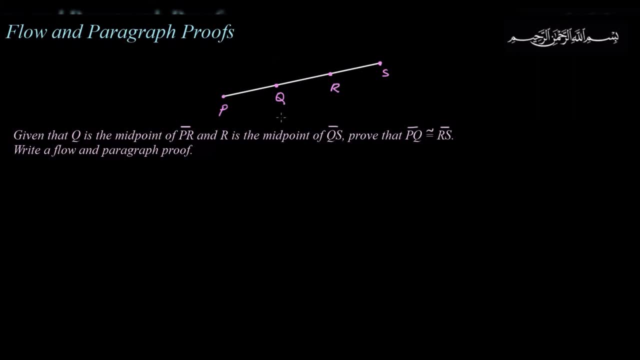 midpoint of PR. So if you're given a diagram like this, you can basically write on it and think to help you think through the problems. So Q is the midpoint of PR. So if Q is the midpoint of this particular segment, it means that this: 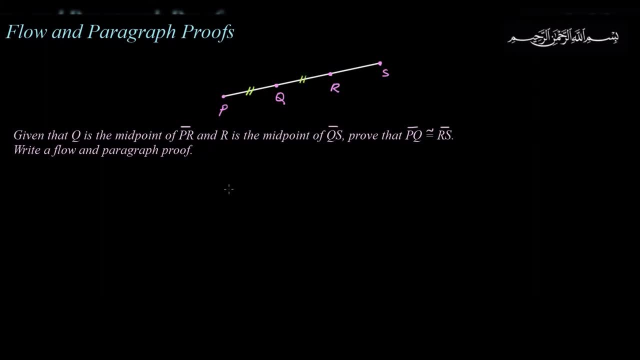 segment PQ is congruent to QR like this, doesn't it? That's kind of what a midpoint is right, And then R is the midpoint. R is the midpoint of QS. So if R is the midpoint of QS, then that means that QR is congruent to RS. I mean, this is congruent to this. 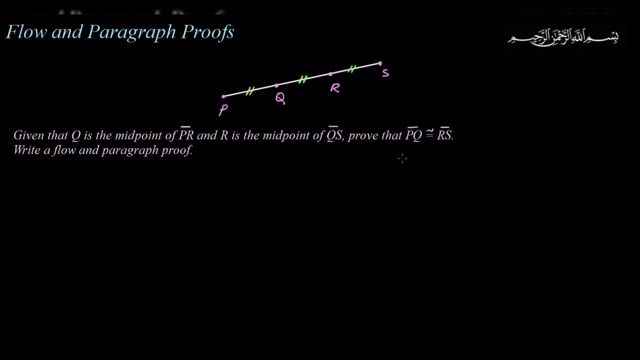 correct. Okay, that means they're all kind of congruent to each other anyways. and then it's easy to see in this visual that PQ is congruent to RS, because if this is congruent to this, then that makes pretty good sense to me. So how do 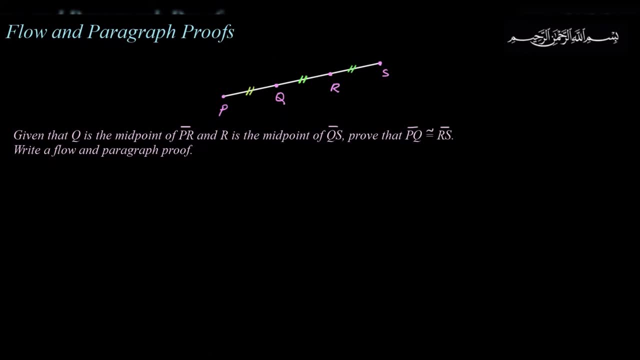 you write this as a flow proof. So in the flow proof, if you remember, the first thing we do is we write the given information. So here it goes. So we write the given information like this: given information involved, In this case I'm. 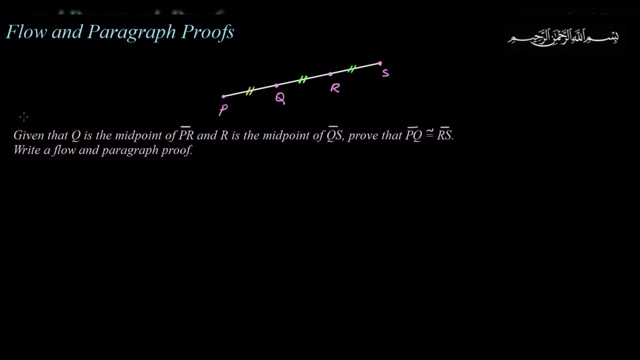 just going to write all of this. So this is all the given information to us. You would rewrite this and then we would say: this is what we are asked to prove. So we asked to prove that. Okay, so where do we start? So let this start with the. 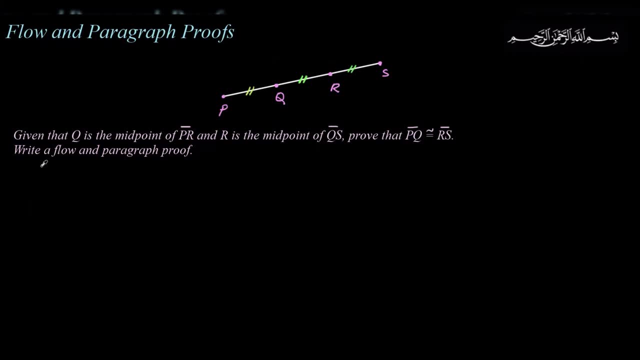 given information. So I'm going to, right now I'm going to write the flow proof. Okay, so here is my flow proof. It's going to. it's going to do quite a certain bit of work. I can tell right now. 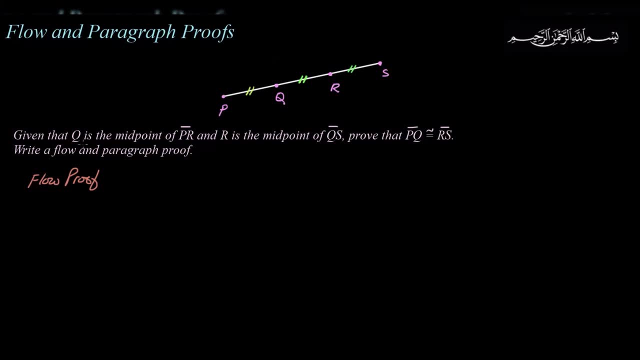 Okay, so start with the given information. Okay, Q is the midpoint of PR, So I just write that Q is the midpoint of PR. Okay, segment PR. So that is given and from. I can also write the second one if I wanted. 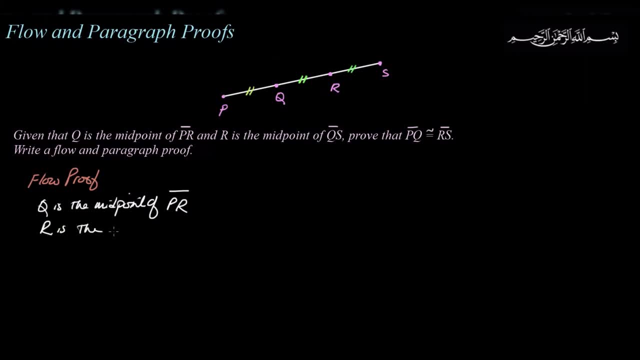 to R is the midpoint of QS. Okay so, and then I can rectangular this. I love rectangularing here like this, and I can say this because this is the given information, So that's given to me. It's kind of funky. 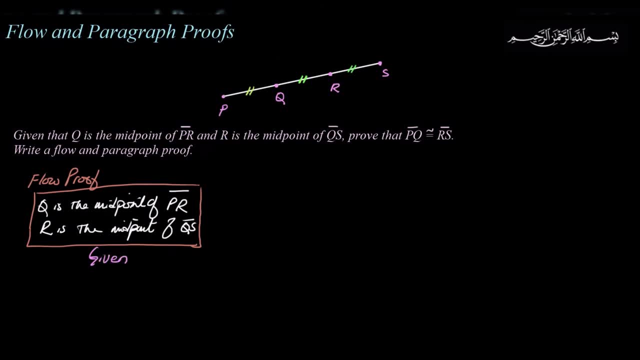 My handwriting is not the best I get it. So, hey, given information. Alright, so Q is the midpoint, So I can say that because that's given information. But my errors are cool. Well, here we go, And from this I can say from: 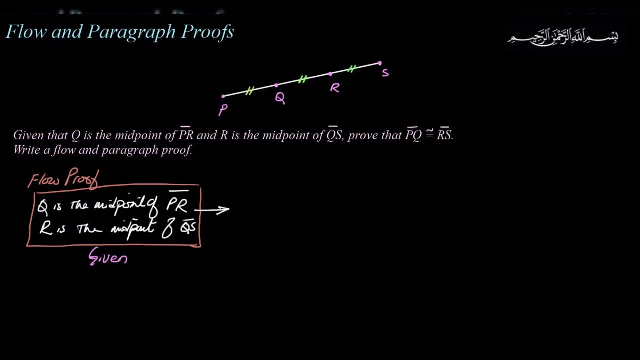 this, I'm going to be able to say the following: Well, if Q is the midpoint of PR, then I can say that PQ right is congruent to QR, Okay. and I can also say that QR is going to be congruent to RS, like this: 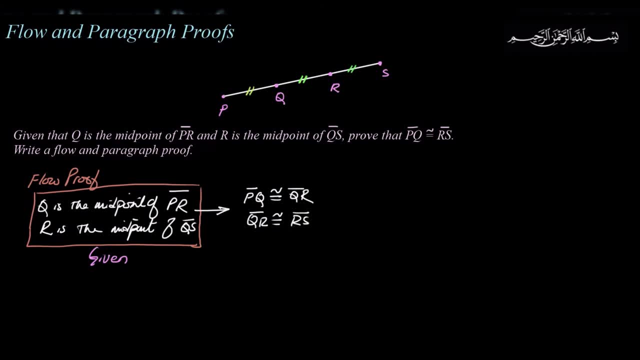 Okay, how? why can I say this? Okay, well, first I can rectangular this, because it's just kind of looking cool, So I have a good, pretty good right. So why can I say this? Because this is from. that's what it means to be a midpoint. This is. 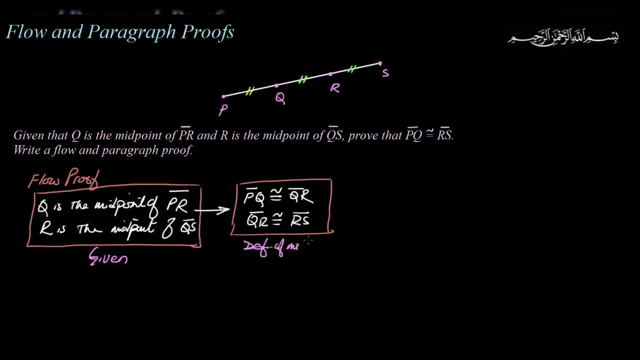 actually the definition of midpoint. A midpoint is a point that divides a segment into two congruent segments, or two congruent segments like this: Okay, alright, so what can I do from here? Well, from here I can say, okay, watch this. This takes a little bit of getting to. 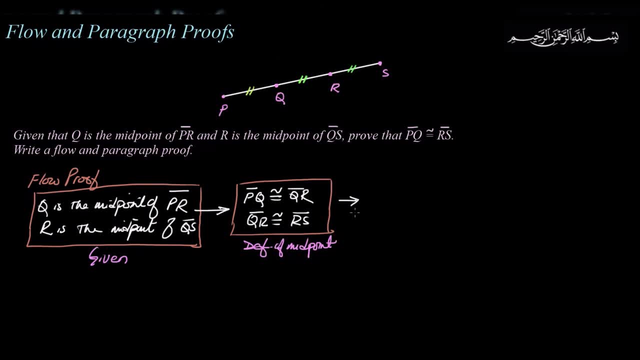 know how geometry proofs work actually. So you have to do this enough times to kind of memorize the logical steps here. So so stay with me. So from here I can say that PQ is equal to QR, PQ is equal to QR, And I also say that QR is equal. 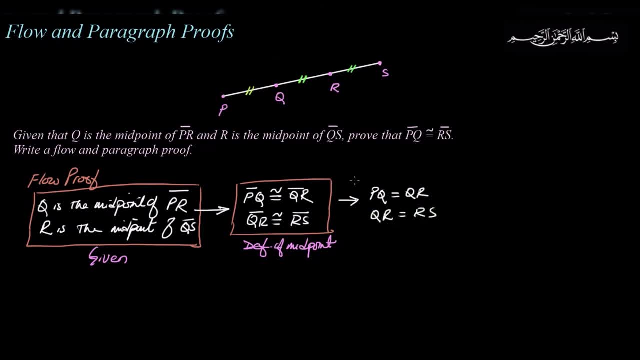 to RS. Okay, and then I can promptly rectangle this like this, And so I just taken the congruent statement and wrote them as equality statement, and the reason I can do this is because this is the definition of congruence, That's. 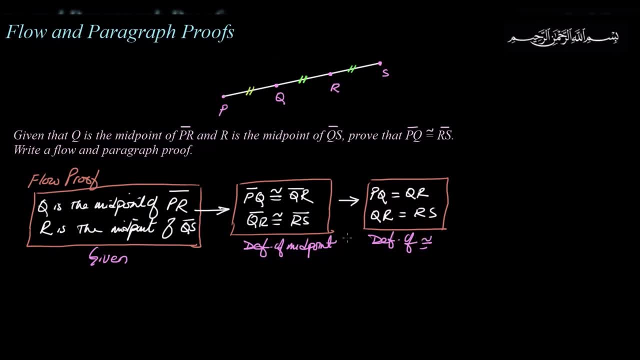 what it means for two segments to be congruent, That their measures are congruent. Okay, now, why do I do this? Because I know only so far. so far, I only know properties of real numbers. Okay, I only know properties, real numbers, I do. 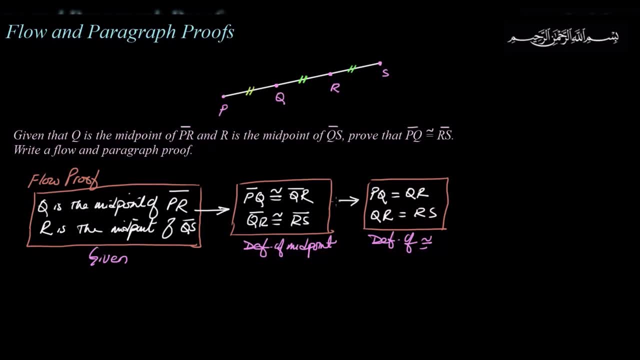 not know properties of real numbers. I just know that real numbers are the properties of real numbers. I just know that real numbers are the properties of real things. yet, okay, so fine, I know this. but now you see, PQ is equal to QR, then QR is. 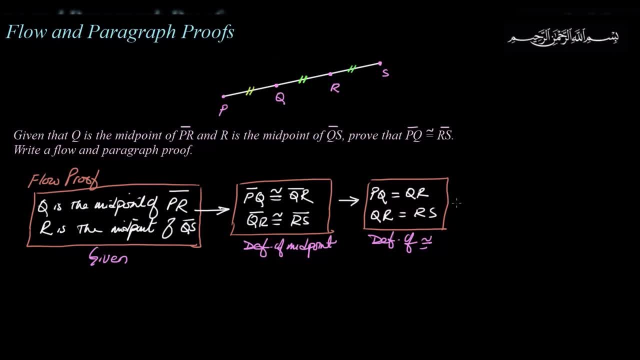 equal to RS. hmm, that sounds familiar to me. if it's A is equal to B and B is equal to C, then A is equal to C, doesn't it? that's like transitive property of equality for real numbers. so I can use the transitive property of equality because 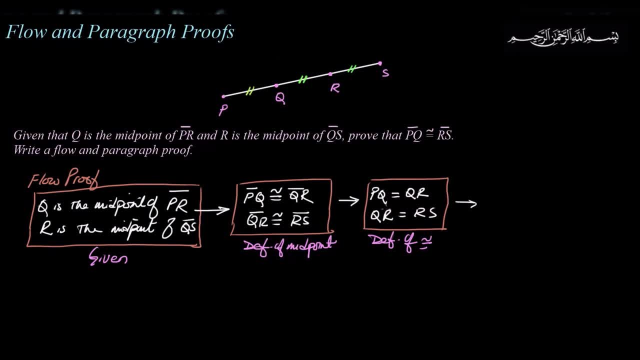 we're talking about real numbers here, because these are measures of segments. so, since this is, since we have something that's overlapping here, something that's common to both of these statements, I can say that PQ is going to be equal in the length of PQ is equal to length of RS, like this, okay, so why can I say this? 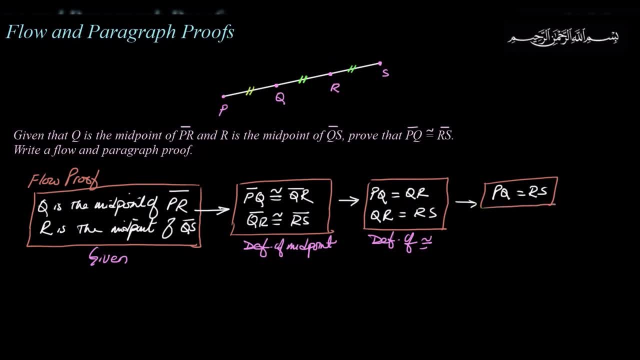 well, because of the transitive property of equality, because of transitive property of equality for real numbers, that's it. that's the transitive property of equality. so, and am I done here? no, we're not done here, because the question asked to prove that they are congruent. it. 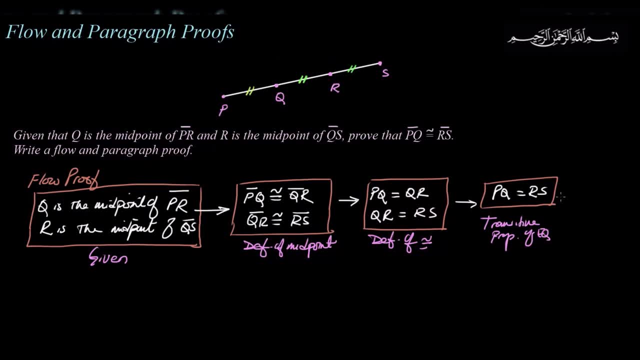 that didn't ask me to prove that they're equal. well, that's easy enough, because then I can say PQ is congruent to RS like this. why? because, darn it, that's the definition of two segments being congruent. so definition of congruent segments: two segments are congruent. 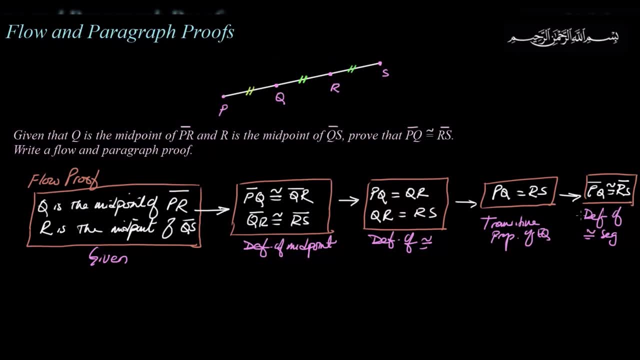 if their lengths are are the same, their lengths are equal. so that's an example of a geometric flow proof. now, what is a paragraph proof? a paragraph proof is really same thing, except you kind of have to type it. I'll write it out. so in this case you, basically you- would put all of this thing in a big paragraph. I'm 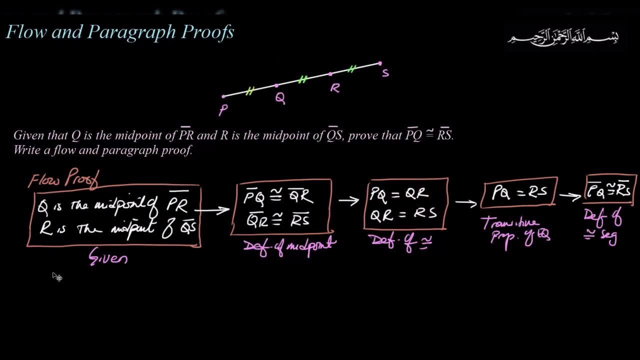 gonna type it up and I'll show you how that goes. okay, so it's no different than the flow proof, but except for the same thing, except it doesn't have the pretty rectangular diagrams and arrows etc. so all of this written out in a paragraph form would be a paragraph proof, and here 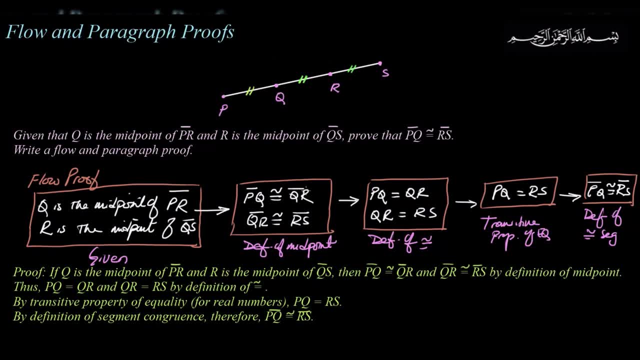 it is. so they have basically typed this whole thing out in words. so I said a proof is the following: the paragraph proof is simply, simply the flow. proof in words I said: if Q is the midpoint of PR and R is the midpoint of QS, so Q is the 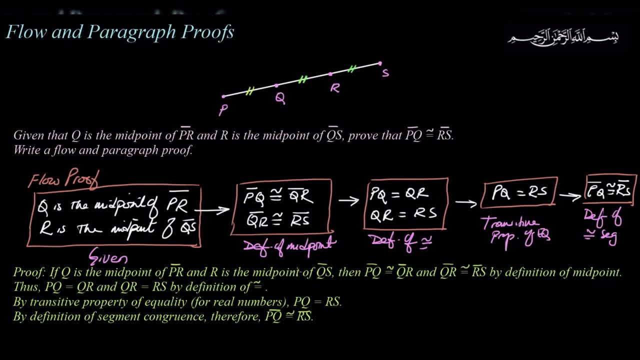 midpoint of PR and R is the midpoint of QS, then PQ is is is congruent to QR like this: okay, this is the, so start out with the given information. if Q is the midpoint of PR, R is the midpoint of QS, then PQ is congruent to QR and QR is congruent to R. basically what I have. 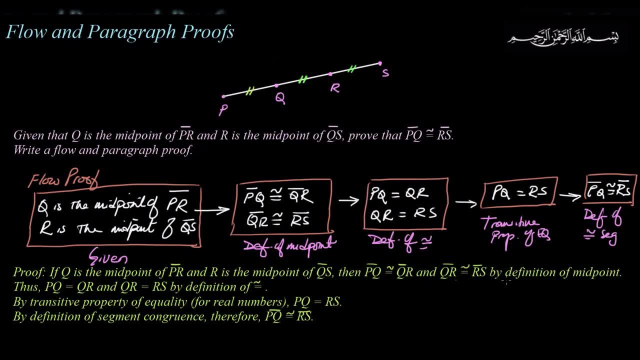 given over here, and the reason for this is the definition of midpoint. just, I have stated over there. from this it flows that PQ is equal to QR and QR is equal to R. This is because of definition of congruence and from there by transitive. 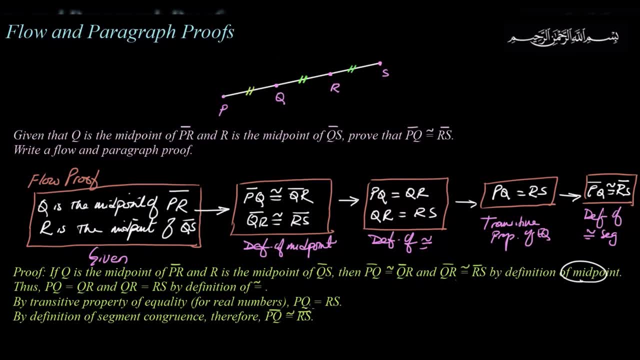 property equality. for real numbers, PQ is equal to RS, and that's this over here. and by definition of segment congruence, PQ is congruent to RS. so this is an example of a paragraph proof. now you can see now the merit of a flow proof because you can kind of visually see this as you kind of think through the. 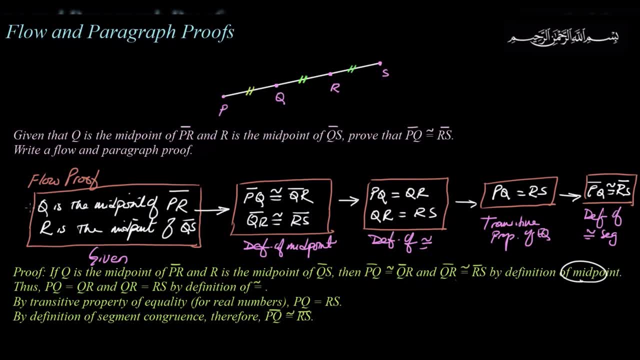 problem. Paragraph proof can get kind of complicated, just looking at it, kind of threatening in a way, isn't it so? but they have their merits. they basically tell the reader, the, how you come to a conclusion. and that's the third form of proof, as I suggested, and let's call it two column proof, which 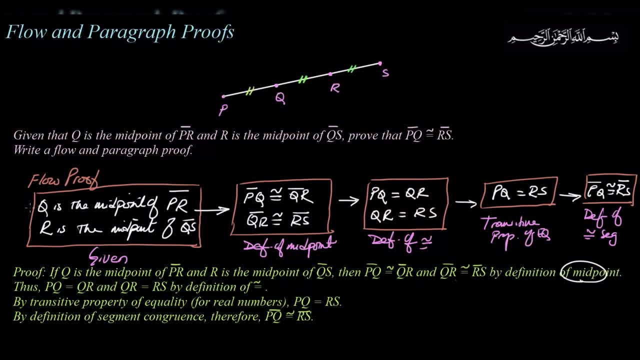 kind of takes the best of both of these and and puts them together. and, inshallah, we shall talk about that in the future. until next time, as-salātu, was-salāmu, was-salāmu, al-hamdu, li-llāhi wa-rahmatullāhi wa-barakātuh. As-salāmu alaykum.